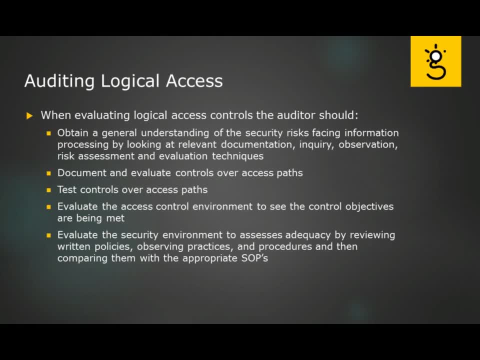 When you're evaluating your logical access controls, you should obtain a good understanding of the security risks that are involved. You want to document and evaluate the controls over the access paths, Test the controls on those same access paths, Evaluate the access control environment to see if the control objectives are being met And also evaluate the security environment to see whether there's adequacy by reviewing the written policies. 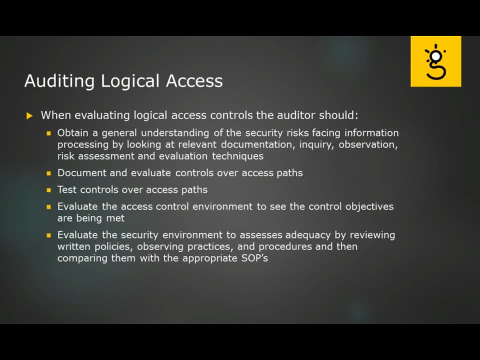 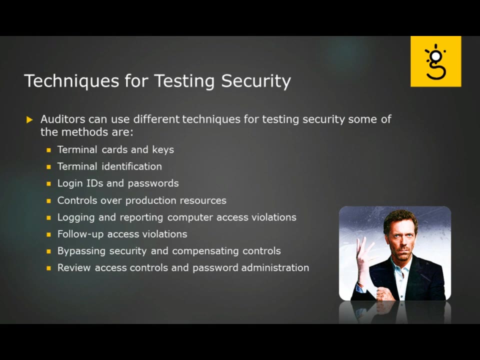 And observing practices and procedures and comparing what you see being done in the field with what you have in the standard operating procedures. Now, there's different techniques an auditor can use for testing security, and some of the methods are things like terminal cards and keys. So let's try that out. Let's take those keys or cards and try them on the things that they're supposed to be authorized for. Try them on those that they're not. 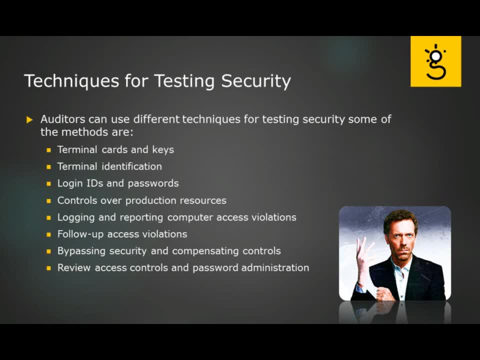 I know I was at this headquarters from- well, we'll just say headquarters- of a large worldwide organization in the southern part of the United States And they gave me a temporary card. and you know, when I'm bored I do my own little audit. I walk by and I see what doors I can get in. 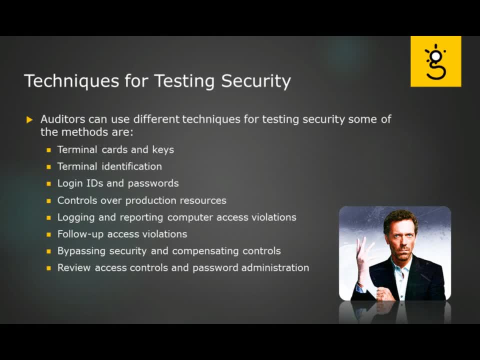 And I've told this story. I think already that I found the one room that I was pretty sure was the network operations, because that was the only door not labeled And that was the only door my key card didn't work. But you know, that's what we're doing, right? I was trying them out. 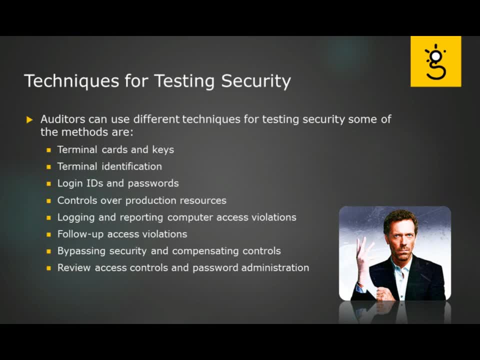 See if they work where they're supposed to and if they, you know, don't work where they're not supposed to work. Same with terminal identifications and login IDs and password, trying them out. Look at the controls that you have over your production resources. 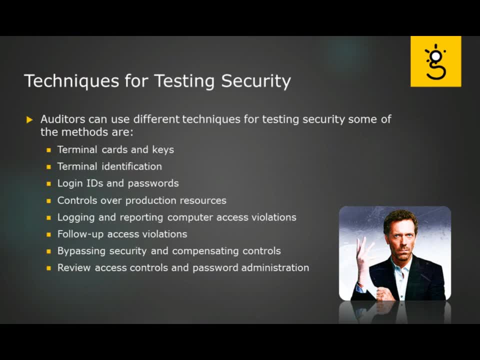 View the logs and reporting to see if a computer access violation shows up. Try to create some. make sure that it's happening, Look at the follow-up that's done on any access violation And if you can bypass security, are there complications.